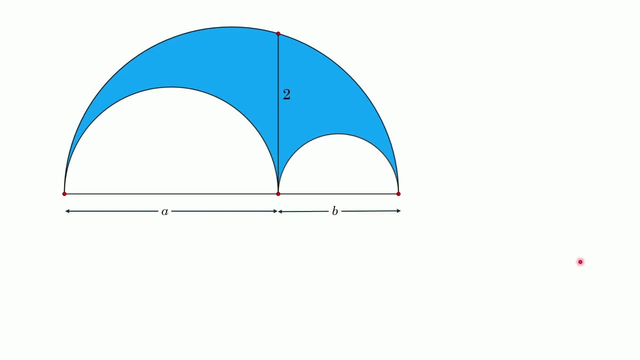 diameter of A and the smaller of the two has the diameter of B, right? So we're going to name those and that'll allow us to even talk about the radius and diameter of the biggest semicircle, right. So the area is one half pi? r squared. It's half because we have half of a circle. Now the radius: 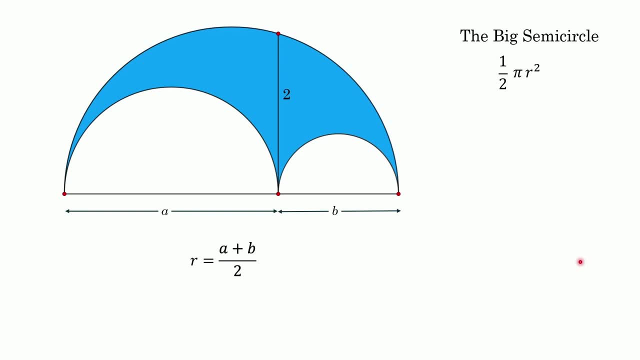 for the big semicircle. well, that would be A plus B divided by two right. So the diameter would be A plus B divided by two. That's our radius. So let's go ahead and plug that in. Here's what we. got. Let's go ahead and clean up that half. So let's go ahead and plug that in. So let's go ahead and plug that in. Here's what we got. Let's go ahead and plug that in. Here's what we got. So let's go ahead and. 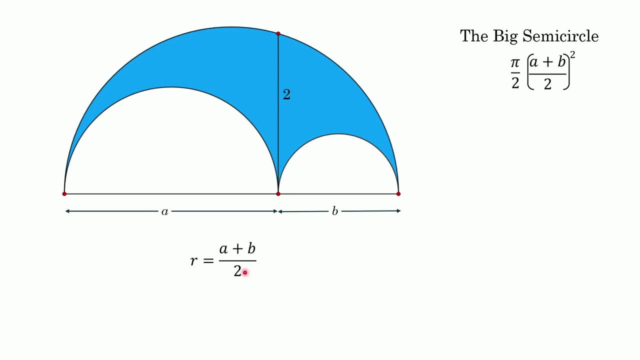 half of pi. so pi over two times quantity A plus B divided by two squared. That would be the formula we're going to use for the area of the largest semicircle, And from that we will take away the area of the smaller two. So let's talk about those, shall we? Now the semicircle we'll 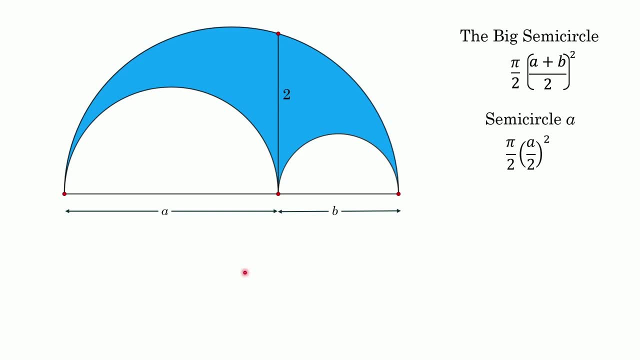 call A with the diameter of A, So you take its radius, which is A divided by two, you square it right And then times pi over two, So pi? r squared half of it right. Pi over two, So pi. 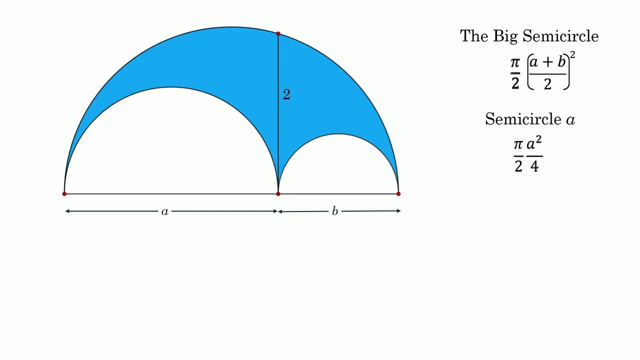 over two times A squared over four. Now, there's a reason. we're going to leave it like that. We're going to do some simplification So we could do, you know, pi A squared over eight. We're going to leave it as it is And we're going to do the same treatment for the smaller semicircle, right. So 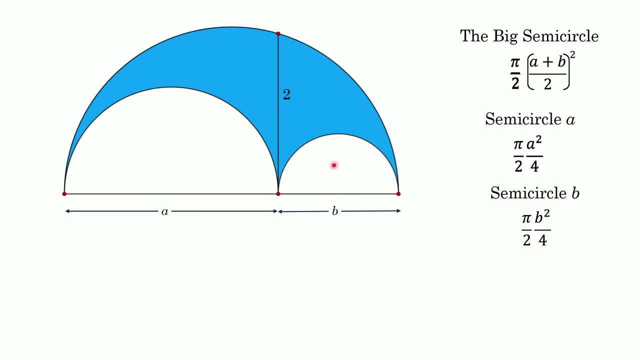 its radius would be half of B. Pi r squared would be the whole circle. We have half of it, So half of pi B squared over four. All right, Now, this is how we said we were going to do it. The larger 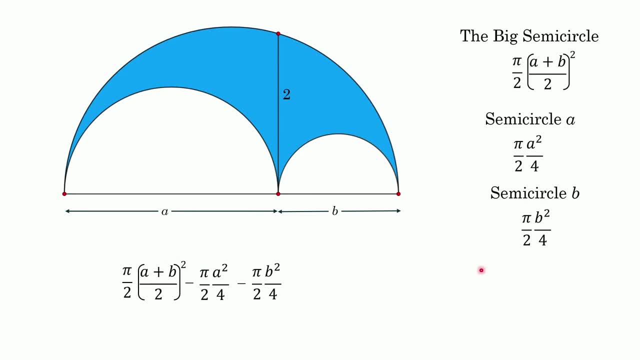 one minus the smaller two. right Now, when we look here, we actually have a common factor of pi over two that we can factor out, And here's what we have left. So that's kind of cool. And A plus B over two squared would of course be A squared plus two, AB plus B squared over four. So we're 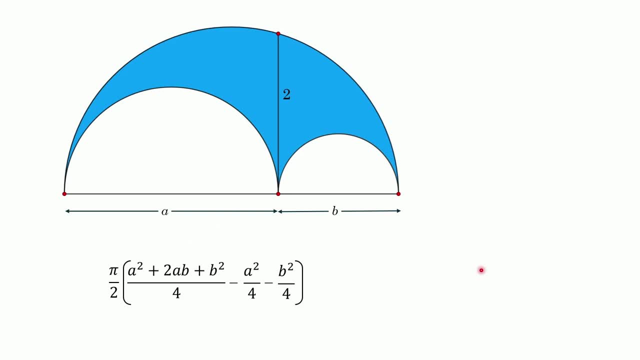 going to substitute that in over there. make ourselves some room. The denominator is four for all of them, So let's go ahead and put them all over four And we're going to rearrange so we can do some simplification: A squared minus B squared over four. So we're going to do some. 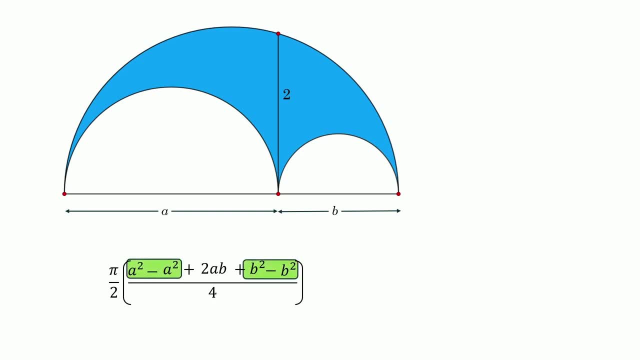 A squared is zero, B squared minus B squared is of course also zero. So what we're left with is, inside the parentheses, two AB over four, So pi over two times two AB over four. That would be the area of the shaded region in blue. Let's go ahead and reduce those twos. Those reduce, And 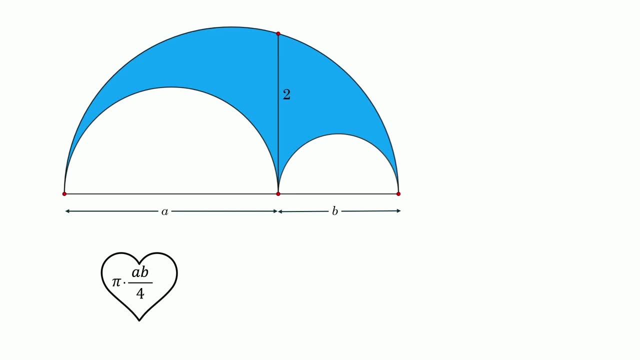 what we have is pi times AB over four. All right, That's pretty cool. Not quite good enough yet, because I would like to know what AB is. So let's explore this distance Two And see if we can come up with a numeric value of AB. All right, Now if we took the two. 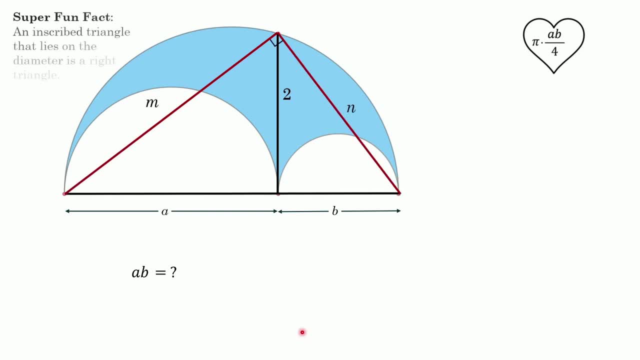 endpoints of the largest semicircle and made a triangle with a base. it would be a right triangle because you know it's inscribed triangle. It lies on the diameter, So that vertex up here would be the vertex of a 90 degree angle. So we have right angles, We have triangle MNAB. That's what. 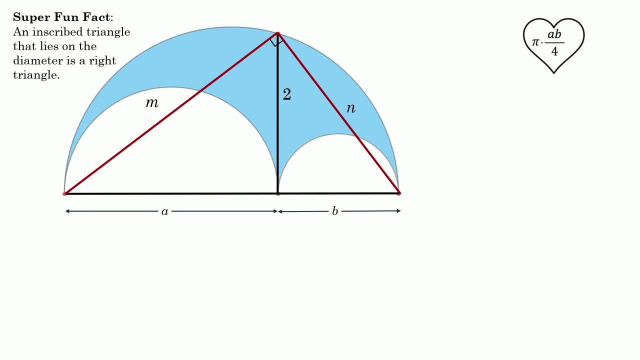 we're going to call it right here. Right, So that's a right triangle. That's pretty good. We can do all kinds of stuff with right triangles, And inside of this right triangle we have two other right triangles- Right, Let's see right over here and here. So, because we have a right triangle, 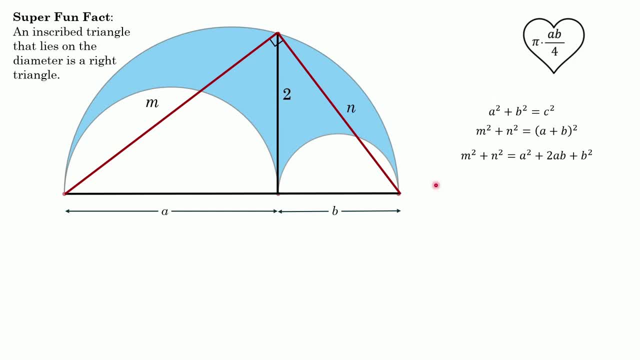 let's do the Pythagorean theorem: A squared plus B squared is C squared. So C squared, we're going to say, is this side And this is A, This is B. So M squared plus N squared equals right A plus B. 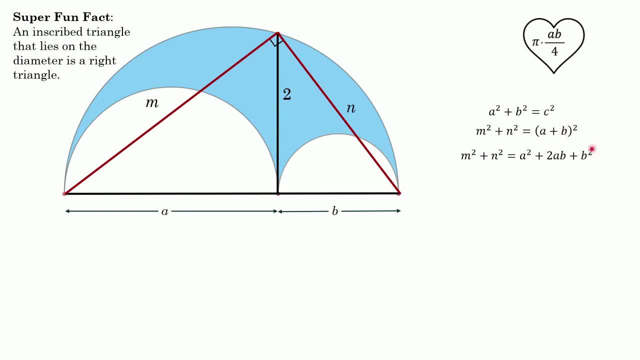 squared, A plus B, quantity squared is A squared plus two, AB plus B squared. All right, That's pretty cool. Now let's do the Pythagorean theorem for this one over here. Here's what we've got: A squared plus B squared is C squared. Here, M is the hypotenuse, Two is one leg and A is another. 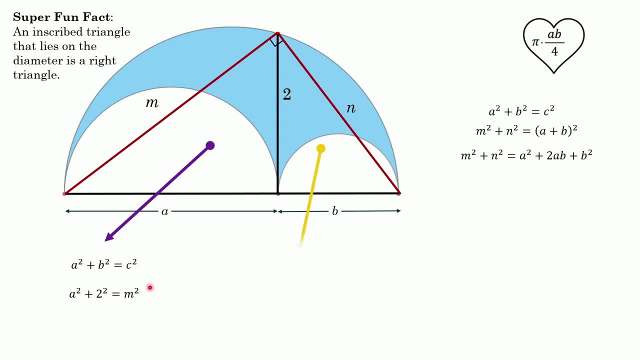 So A squared plus two squared equals M squared. And let's do the same thing over here for this one, Right? If you look at this triangle over here, hypotenuse is N. One leg is two, The other leg is B. So A squared plus B squared is C squared would be: B squared plus two squared equals N. 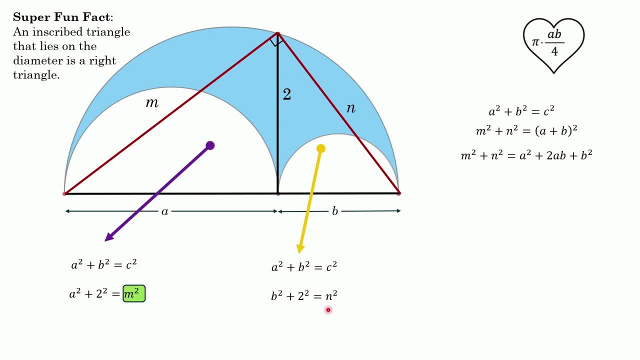 squared. All right, Now we can do some substitution, because you see, we have an M squared here, We have an M squared there. We can substitute those things, And we have an N squared here and here, So we can just go ahead and do those substitutions like this Right. All right, That's pretty cool. So let's go ahead and. 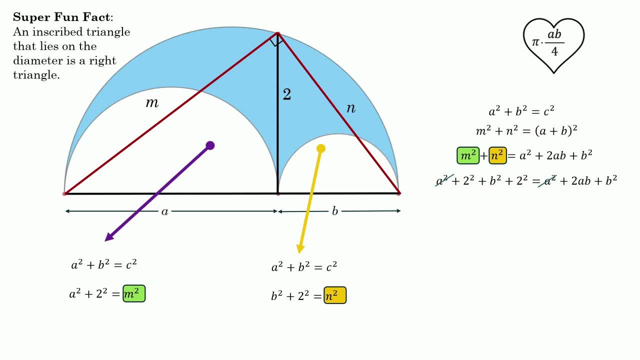 get rid of those so we can start cleaning this up. You can see, we can subtract A squared from both sides. Those will go away. We could do the same thing with the B squared. So what we have is two squared plus two squared equals two AB. Well, two squared is four, So that's four plus four. 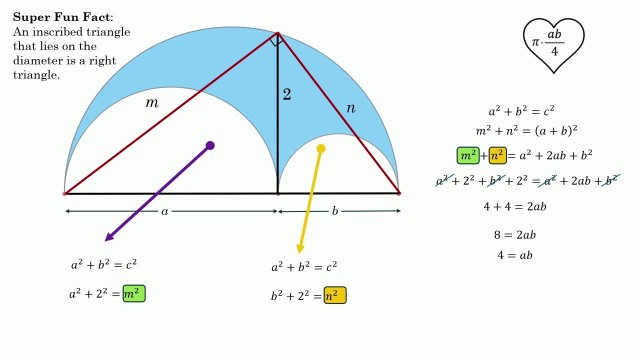 eight equals two AB, So AB equals four. That's pretty cool because our whole thing was AB over four times pi would be the area of the shaded region. So if we plug that in man, that's four over four, which is one. One pi is the area of the shaded region. I think that is super, super cool. 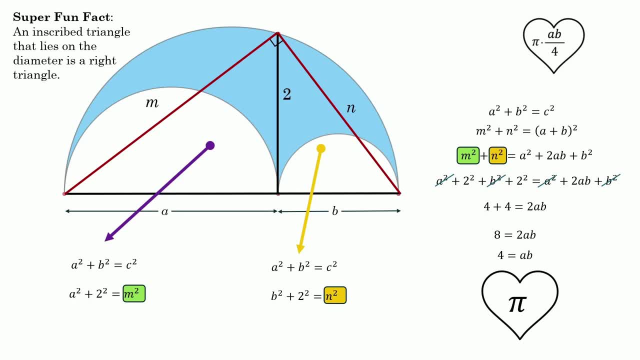 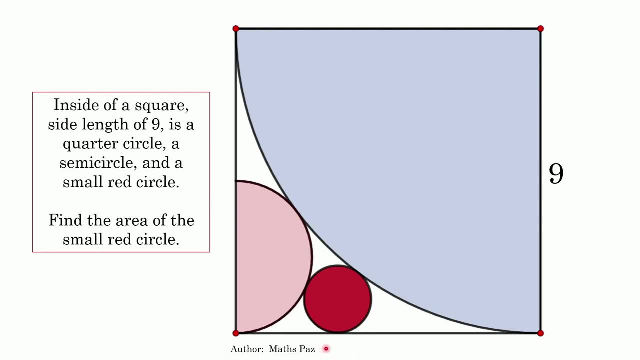 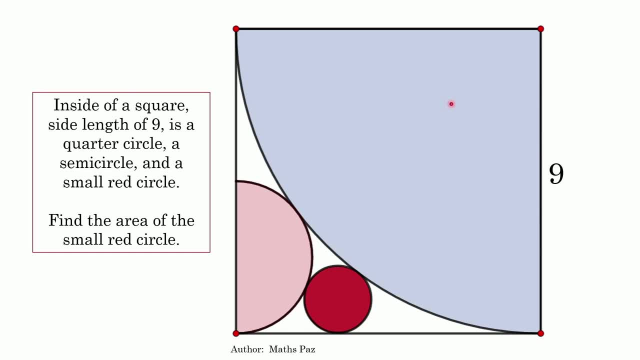 of the mathematical ideas, which I think is kind of a neat thing. I went ahead and recreated the picture, but I'll let you watch his video on how to solve it. We've got a square with a side of nine, a quarter circle inside of it, a semicircle over here and this little red circle You have to. 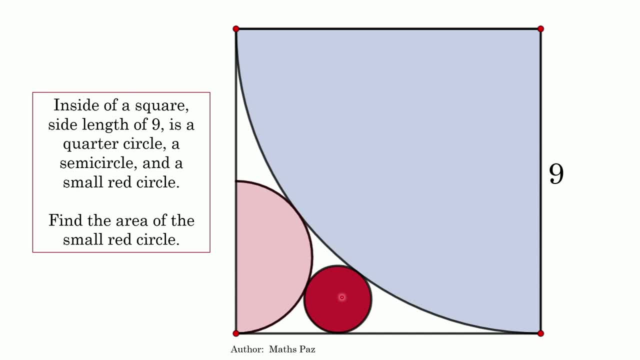 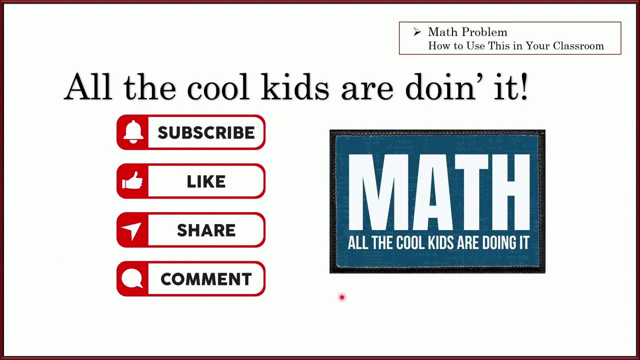 find the area of that little red circle right there. So I'll leave a link to his video in my description below And if you like this video, please do me the kind favor of like, subscribe, share and especially comment. I really love to hear from you guys, Hear what you think. 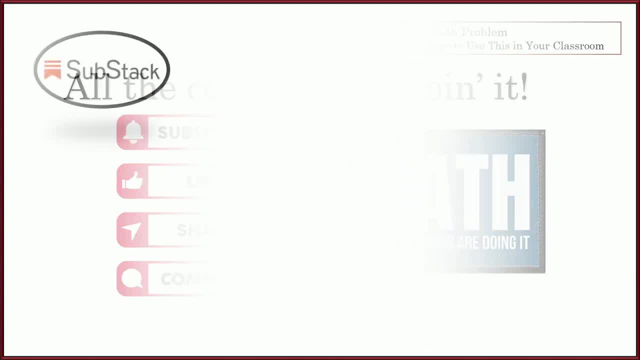 and what you like and what you'd like to see next. And if you like to do a weekly math problem, check out my sub stack. I've got one there just for fun. There's also some resources that are pertaining pertaining to that problem that you can use in your classroom for free, that I post. 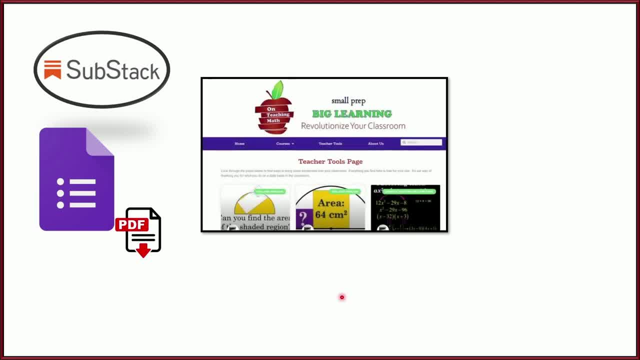 for you. I've got a website on teaching math dot org. all kinds of cool stuff there: some blogs, some resources, a lot of free stuff- And I have a teacher's pay teacher's site. So if you're interested in using some innovative and very easy to use math resources in your 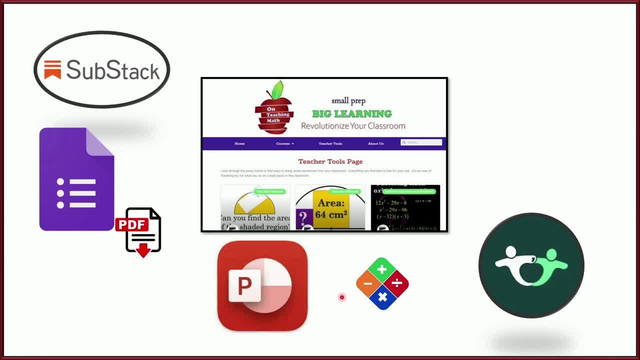 classroom. please check that out as well. I'll leave links to all of that in the description, And until next time, I do hope you have a wonderful day.